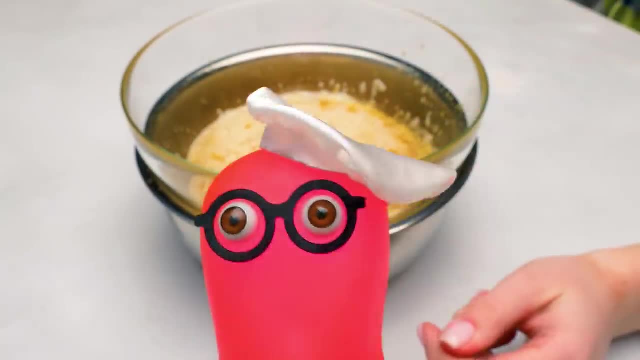 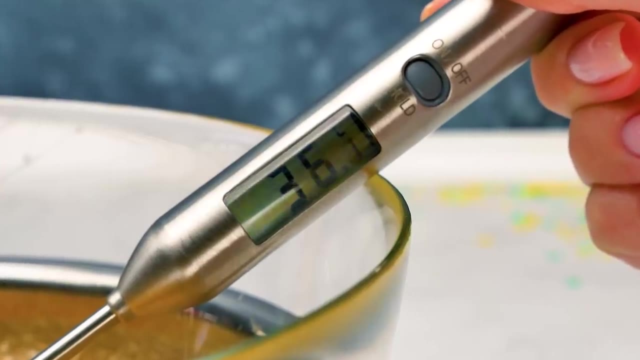 A quick tip: You can place the bowl with the batter on a bowl with hot water. The most important thing is to control the temperature, not to overheat the mixture. The home oven starts with all the sugar at its maximum: Cool, Perfect. Now I'll take the bowl out of the waterbath…. 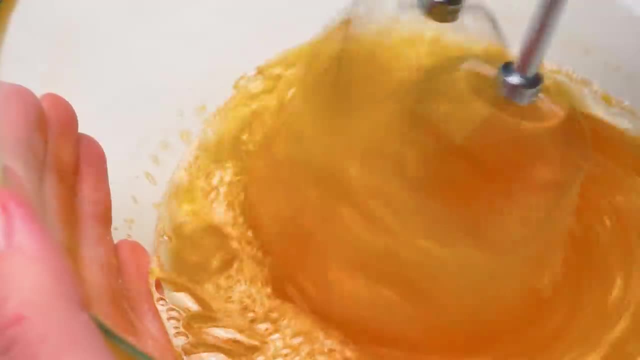 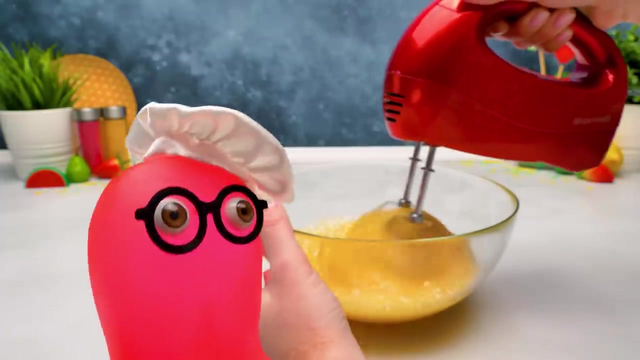 And mix it again in theen. we're pouring the mixture. Do the same for the 너무. yours Look so easy. I think I'll try, Off course, but we need to come here because we can't stop mixing. Well…. 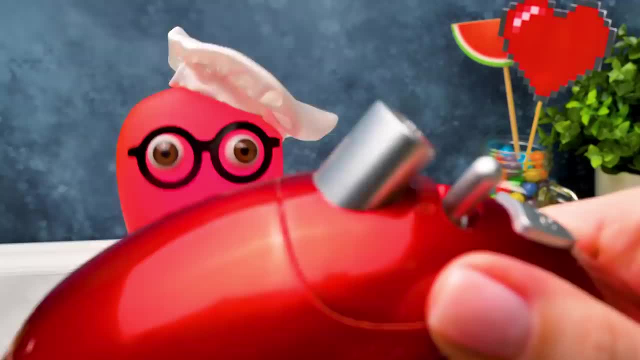 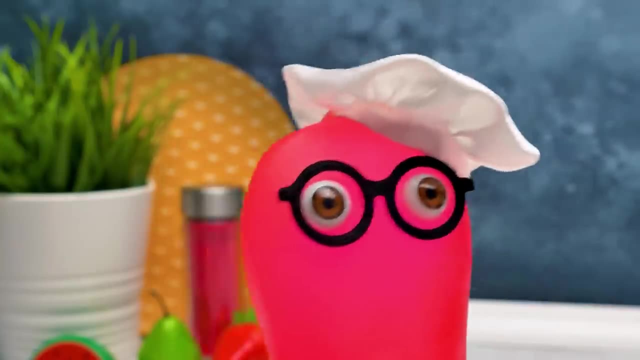 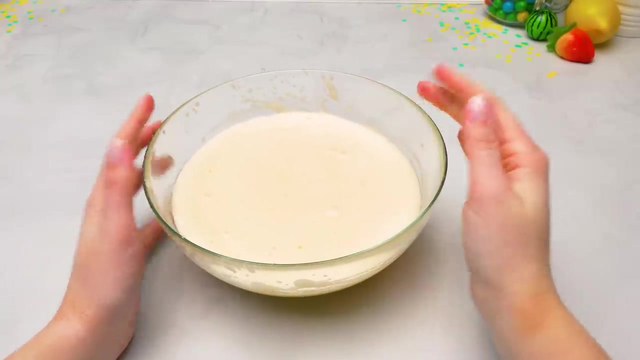 I'm still here to find…. Get away, He-he. Ooh-oh Good, I'm finally here to fix it. high-speed mode: we need to make bubbles. that was close. I have to stay away from those mixers. now we're ready to add some more ingredients. Sammy, get the warm milk. 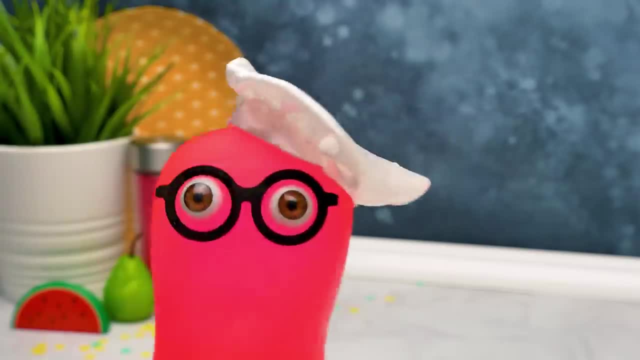 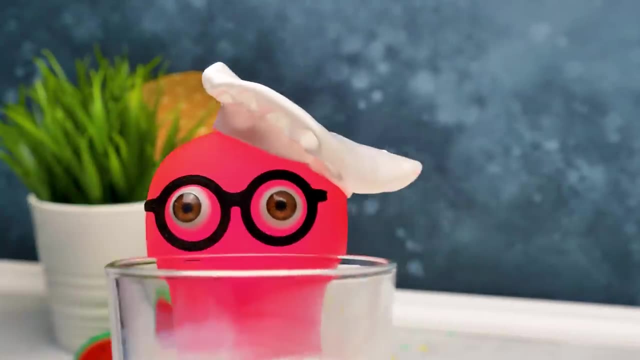 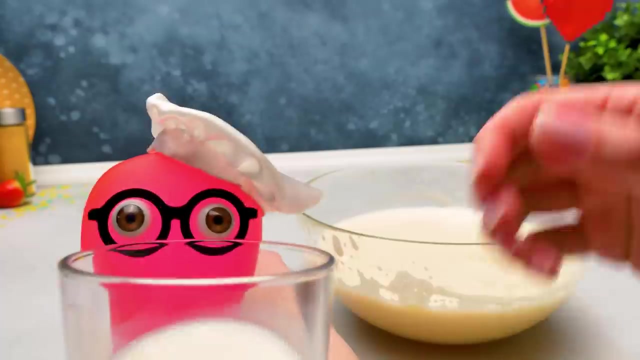 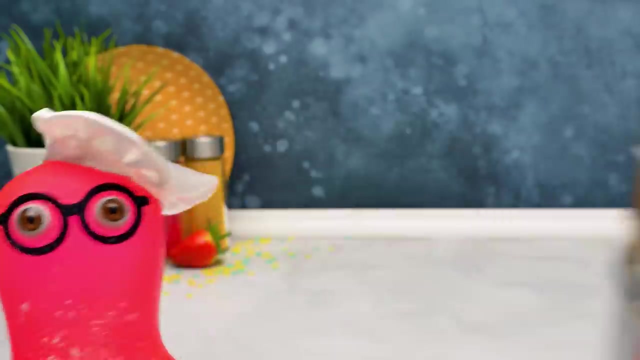 please about that. you know I kind of drank it. I wasn't serious. Oh, Sammy, I was so stressed out. don't joke like that. here's your milk, 50 degrees Celsius, as you ask. okay, here come the 30 milliliters. next we need 95 grams of flour. get ready to be all covered in it. we'll add the. 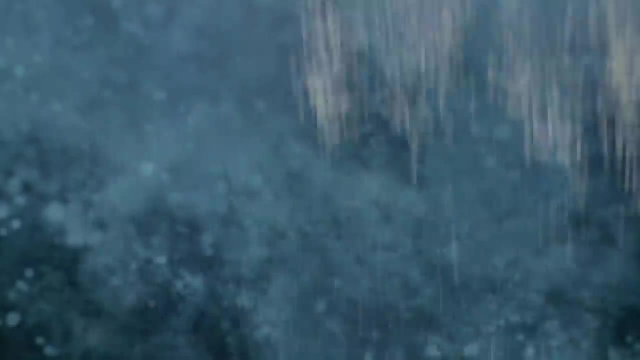 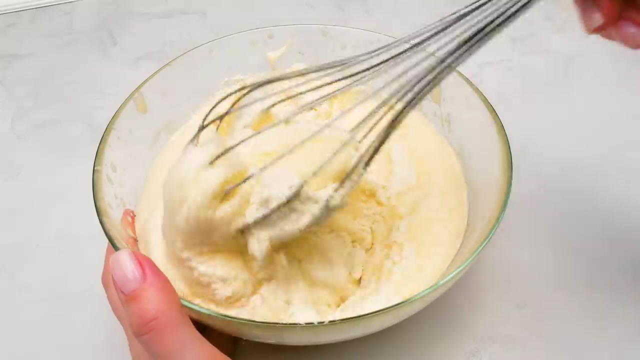 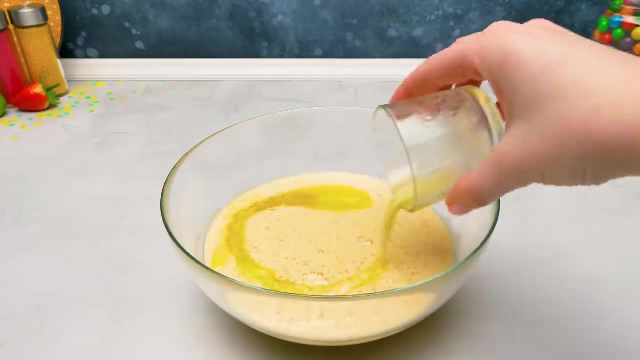 flour to the mixture using a sieve. now we can mix it properly. hurry up. the butter is melted down. what are we gonna do? all right, Sammy, the butter temperature should be exactly 50 thousand degrees celsius. now we're going to add the flour to the mixers. 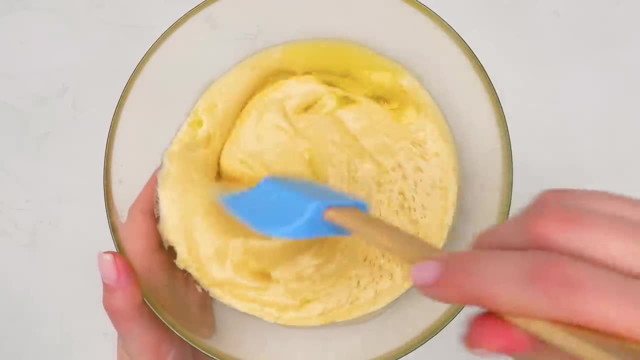 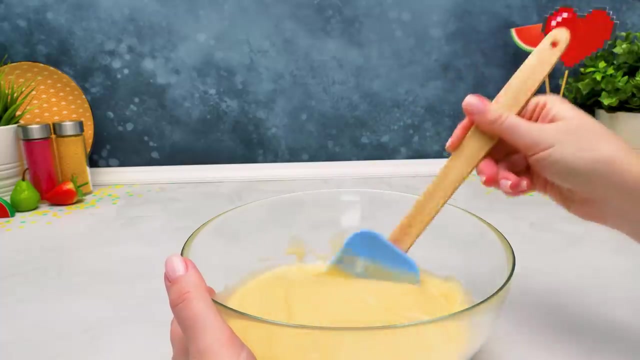 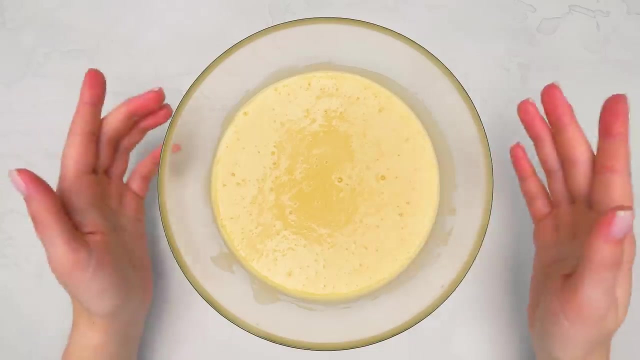 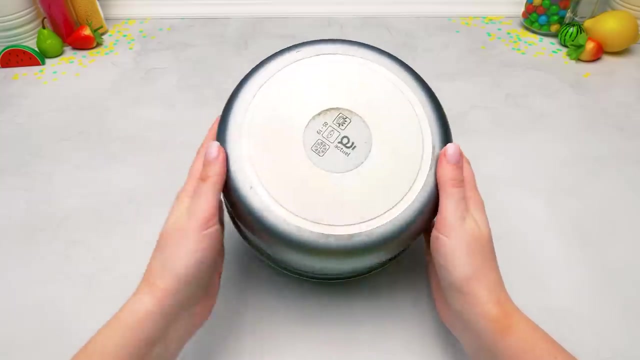 5 to 60 degrees Celsius, guys, we use 30 grams of unsalted butter. mix, mix, mix, mix. again, everything is about mixing stuff. yep good, mixing is the essential part of cooking, do you agree, guys? then give it thumbs up, the batter is ready and we can finally bake it. for this, we'll need fresh-baked Sam is here, Sammy. 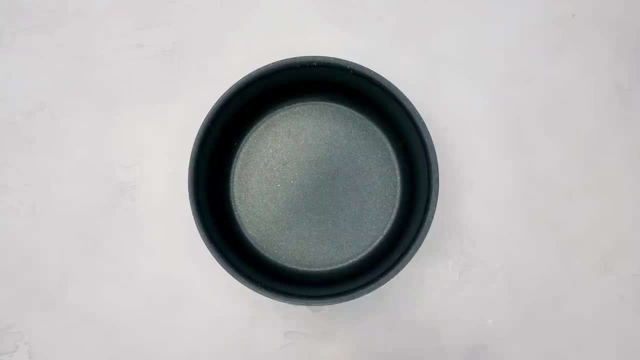 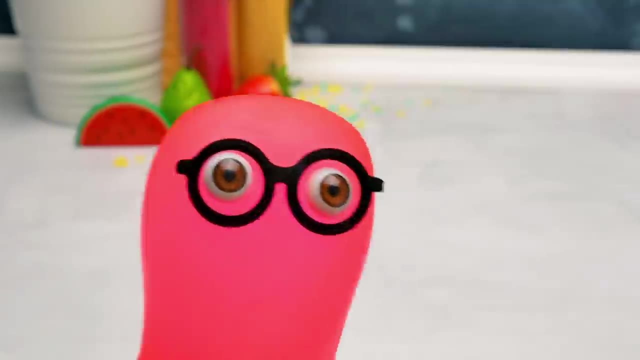 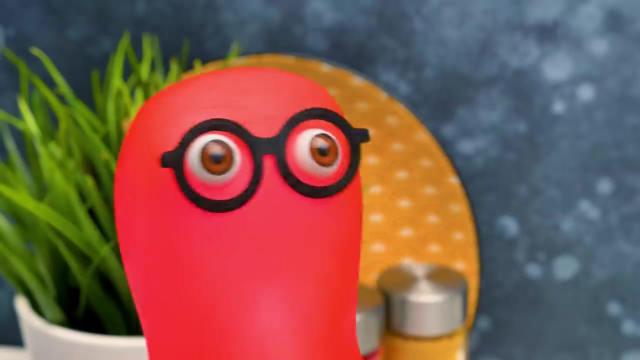 you're full of surprises. by the way, the cake pan size is 15 by 7 centimeters. put baking paper like this. but ah, it already looks so yummy. can I taste it? uh-huh, I know you, Sam, you won't be able to stop. but what are we gonna do next? 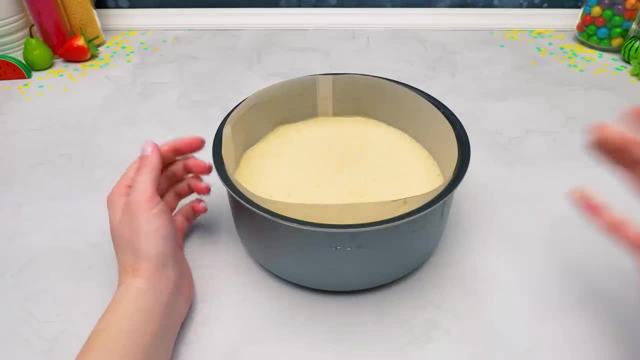 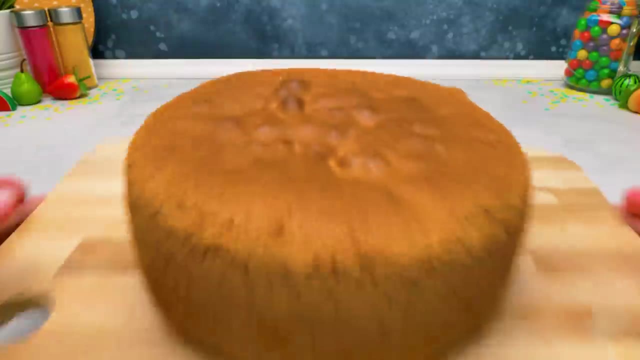 the oven is preheated, then we bake it at 160 degrees Celsius for half an hour to get a fluffy sponge cake. our sponge cake is ready. now we need to cut it into four round pieces. one centimeter thick is the best. one centimeter thick is the best. 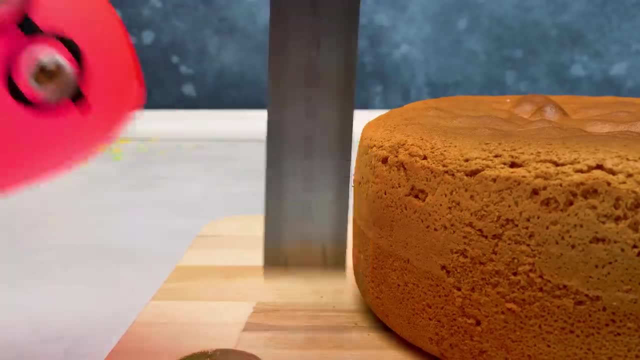 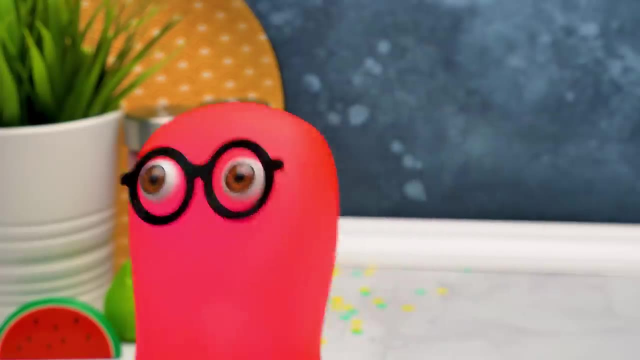 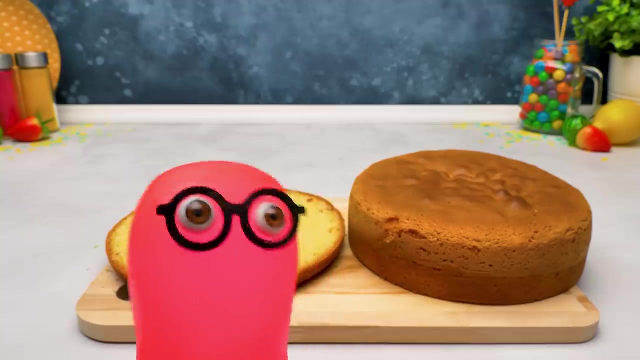 ask an adult to help you with it. the knife is not a toy. we will do it smoothly and steadily with a sharp, long knife. oh, I better not watch it. what if it doesn't come out nicely? don't worry, Sammy, check it out. everything's fine. well, you need three more slices. that's three more chances to make a mistake. I 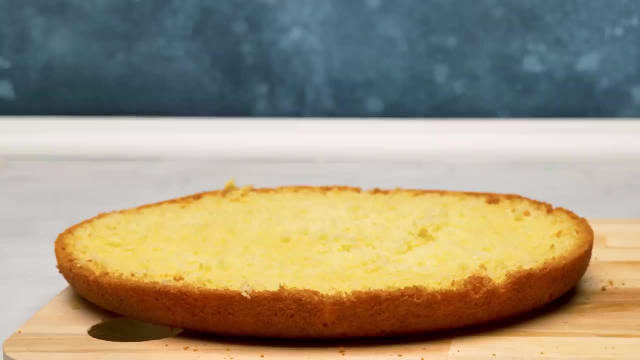 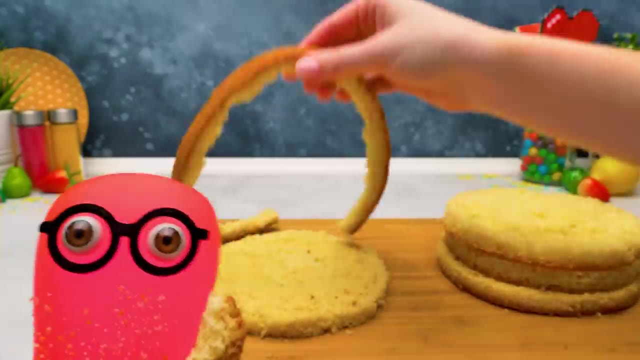 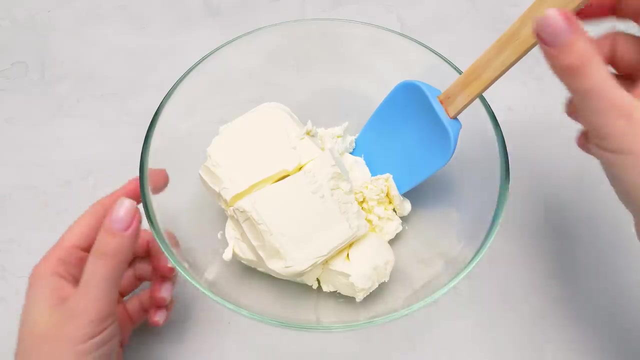 promise you I'll do it so fast you won't even have time to get scared. this sponge cake is so yummy- hail the great tippy-dum- that we don't need the edges, and I can eat all of them. in the meantime, I prepared 270 grams of cream cheese for our special frosting. it's very important. 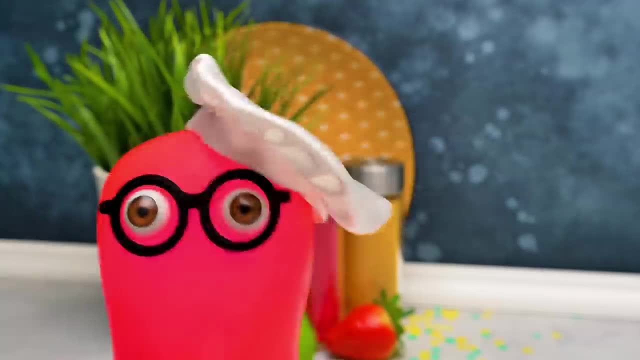 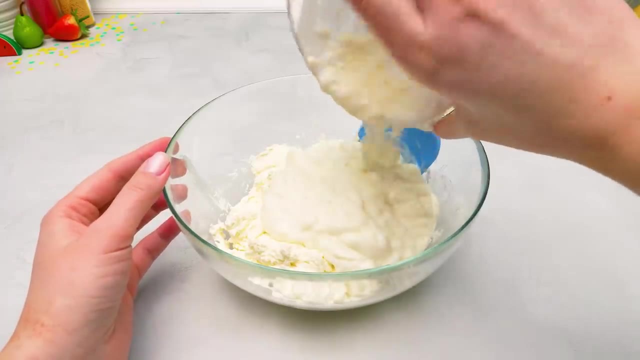 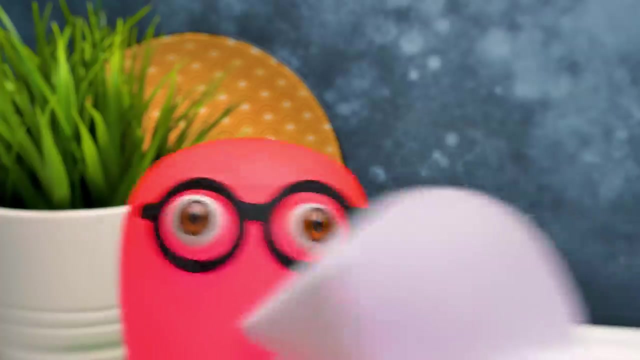 for this type of cake. so let's mix it properly. don't be afraid, cooking is fun, just enjoy your time. the cream cheese is ready and we can add 160 grams of unsweetened yogurt to it and mix it all again. add more sugar, no sugar, no cake. all right, all right, all. 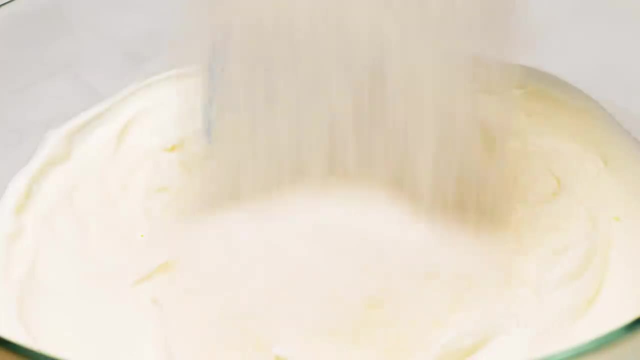 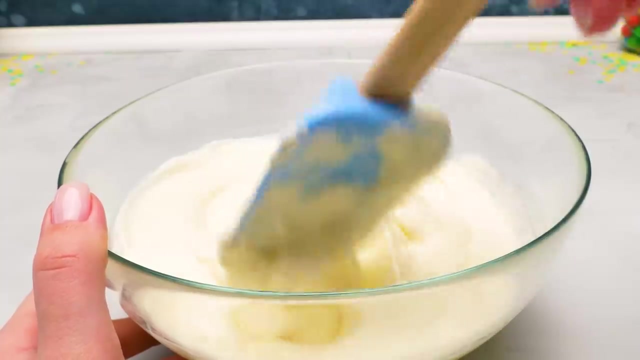 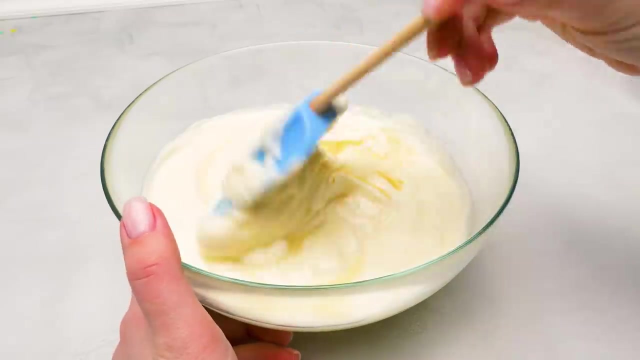 right, 95 grams of sugar for the frosting. is that enough for you? pretty much, mix it well, sue, I'm watching. you don't be harsh on me, chef. Sam, I'm doing my best. now we add 5 milliliters of vanilla extract and 10 grams of lemon juice and mix everything up. it looks like today. 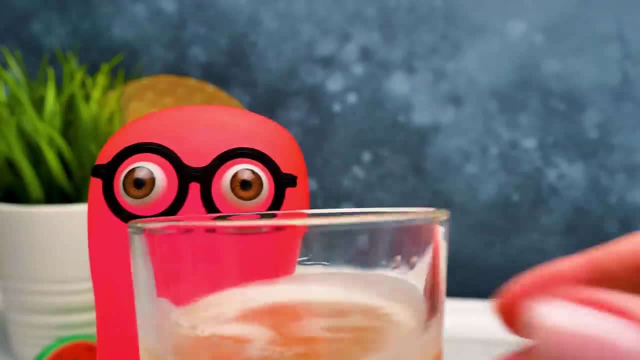 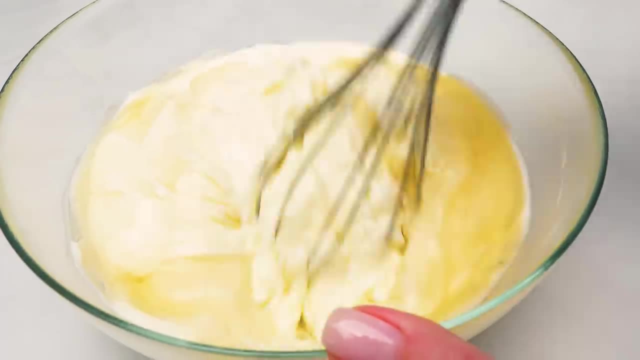 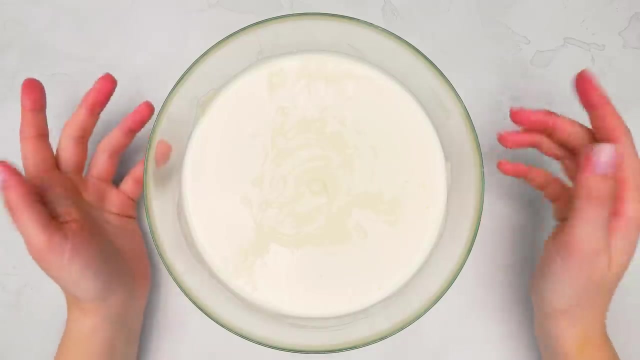 I'm mixing a lot. why do we need to add melted gelatin into the frosting? sounds odd. melted gelatin makes the frosting thicker. you'll need 7 grams of powdered gelatin and 35 grams of water. the frosting isn't done yet. the final step is to add 50% whipped heavy cream. 150 grams is enough. let's mix it well. 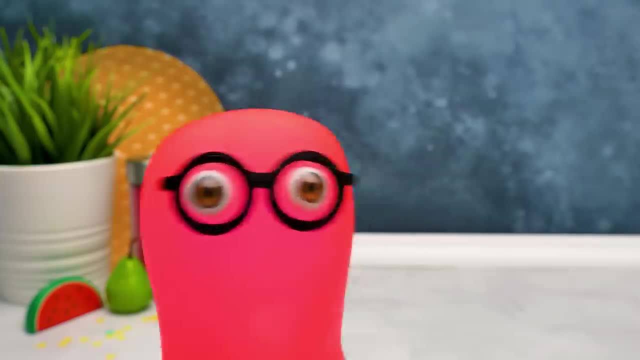 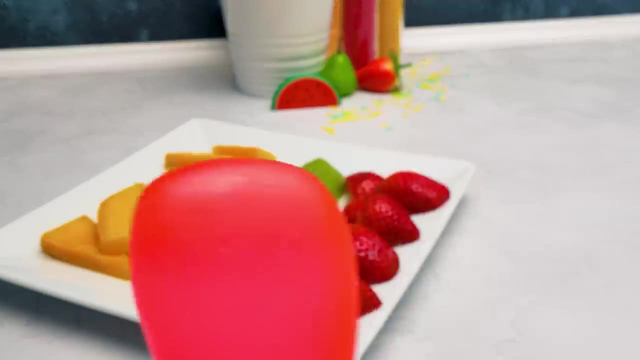 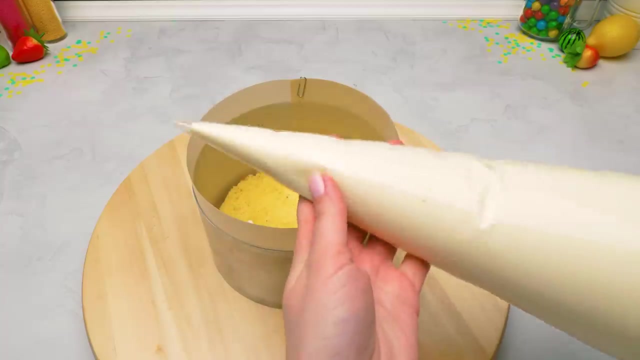 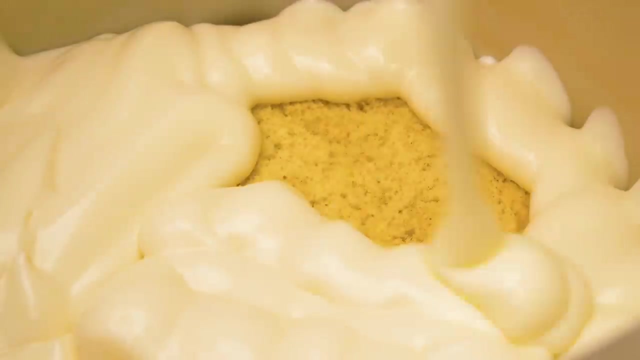 for the last time. no, I need to distract myself from the frosting guys. we can finally put our cake together. we'll need this pan. I've already cut a piece of the cake inside and now let's add 1 quarter of the frosting. we need to spread it evenly, like that. 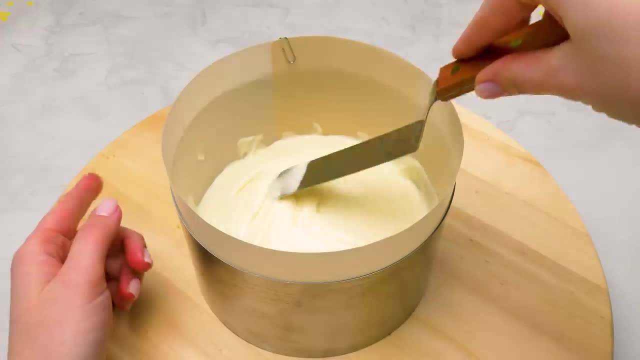 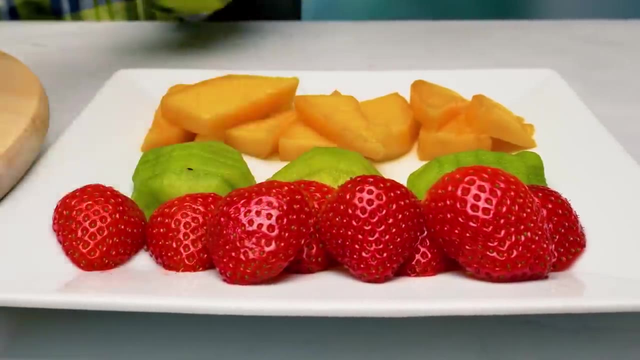 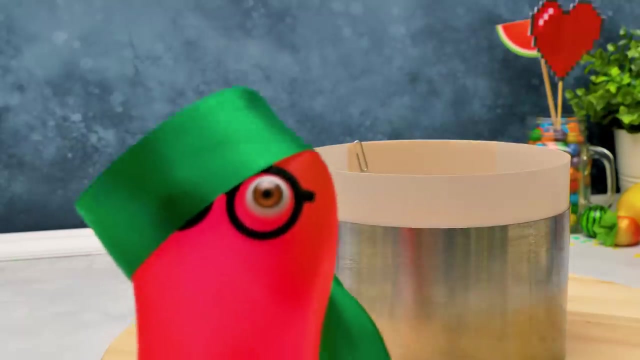 how is everything going? I can't see much now. Sammy, why are you blindfolded? you'll miss the best part. we'll put different types of fruits on each layer. this one will be strawberries. I have to do it. the cake is so tasty I just can't find just a little peak. wow. 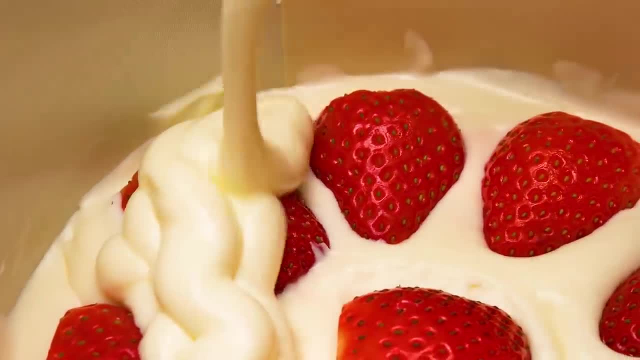 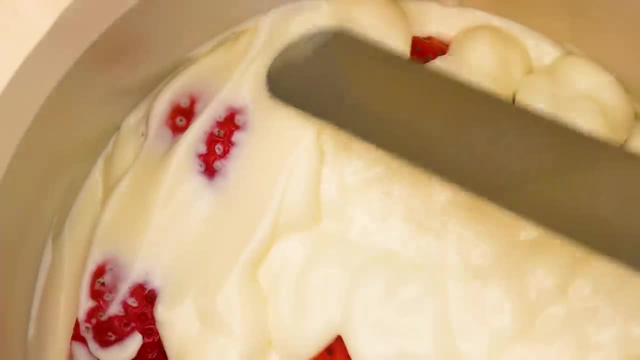 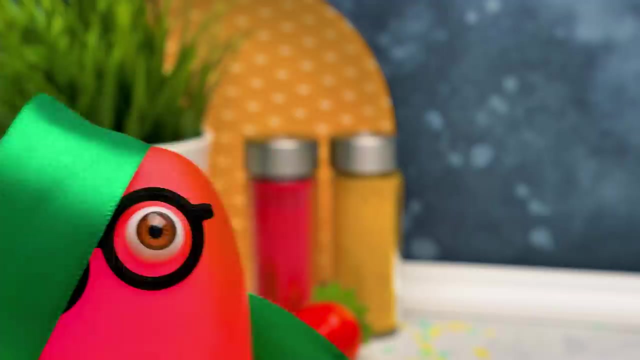 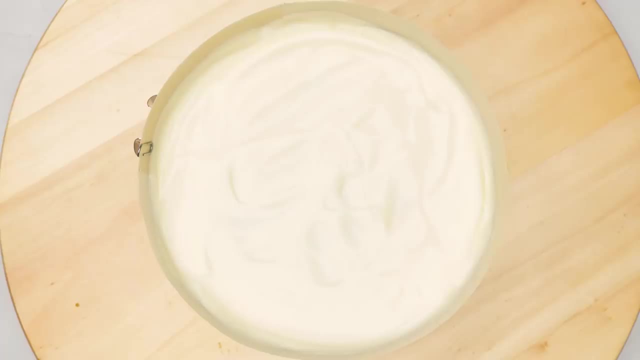 we need to repeat these steps again. the next layer will be with mango, and now we need to repeat these steps again. the next layer will be with mango, and now we need to repeat these steps again. the next layer will be with mango, and now the final layer with kiwi. wait, there were. the next layer will be with mango and now the final layer with kiwi. wait, there were. the next layer will be with mango and now the final layer with kiwi. wait, there were definitely more pieces of fruit. sorry so my. the final layer with kiwi. wait, there were definitely more pieces of fruit. sorry so my. 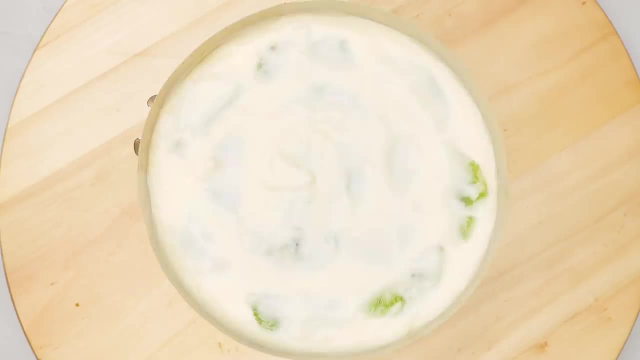 the final layer with kiwi. wait, there were definitely more pieces of fruit. sorry so. my passion is stronger than me. huh, it's done. definitely more pieces of fruit, sorry so, my passion is stronger than me. huh, it's done. Now let's put it in the fridge for two to three hours. 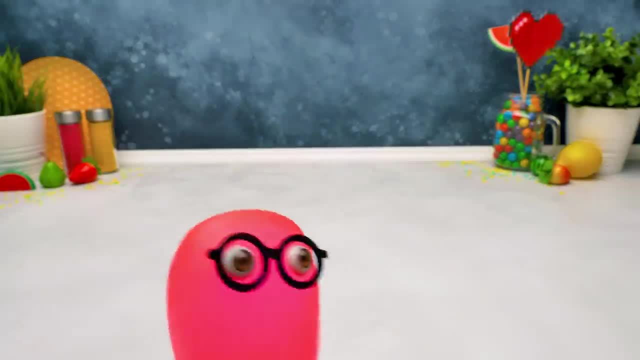 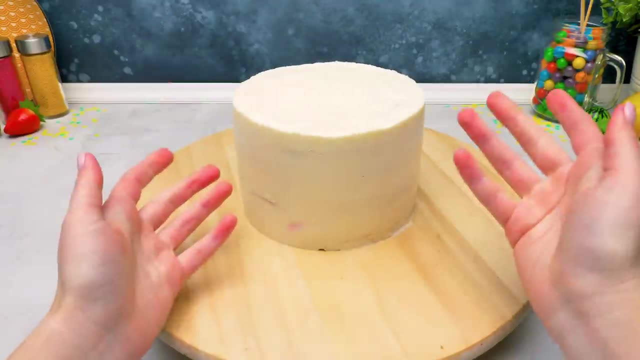 Sammy wanna have more fruit? Yeah, do we have more mango And strawberries? I can't have enough. Three hours finally passed and this is our cake. Delicious, isn't it? Sue? I'm not gonna trust you anymore. You promised me a jelly cake. 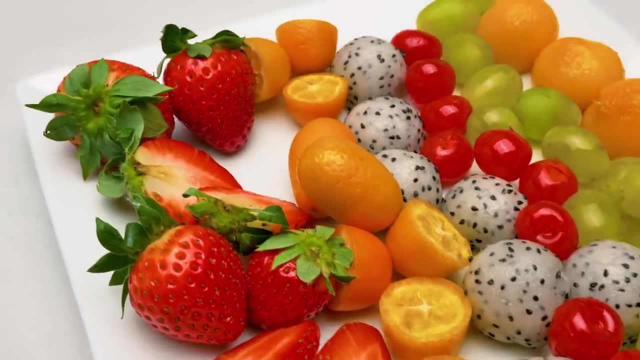 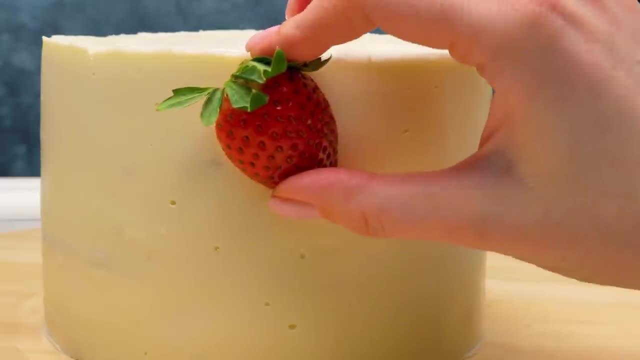 Yeah, we have one more stage, So you just need to be a little bit more patient. I take my words back then. Oh, oh, I think I ate too many fruits. I can see them everywhere. That's because they are everywhere. 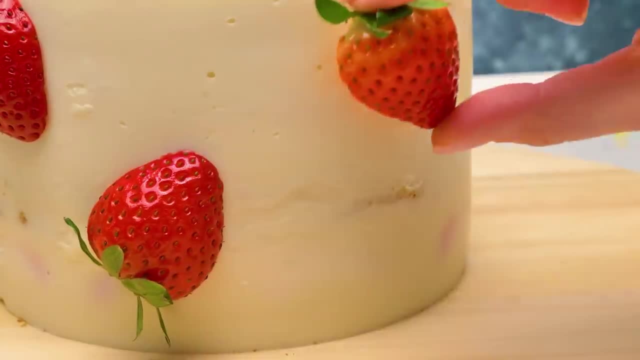 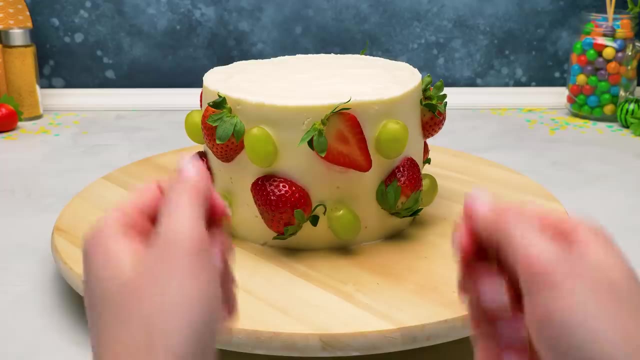 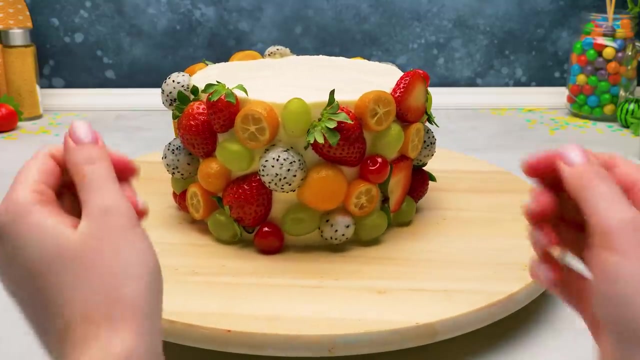 These ones will cover the cake. We'll start with strawberries again. I like them, especially with cream. Sue, I wanna try too. Let me attach these grapes. Nice job, Sam. Now let's add the rest of them. Wow, looks juicy. 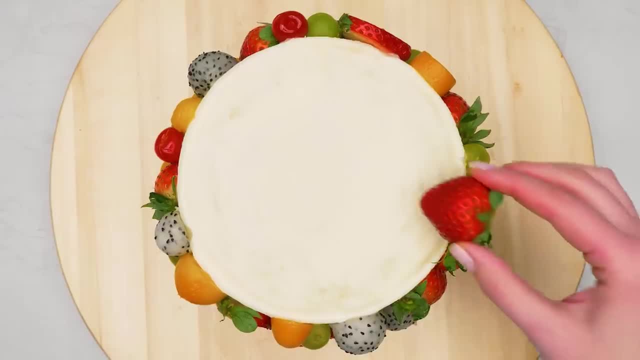 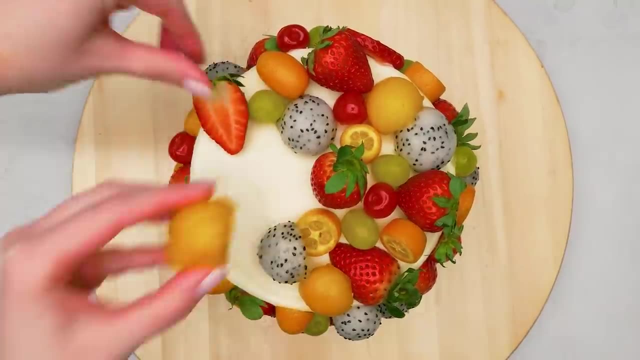 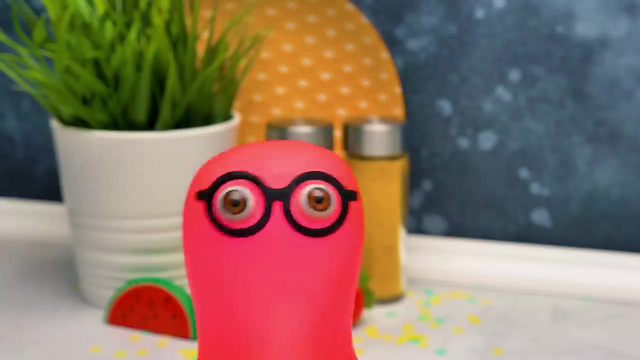 Guys, only the top remains. I'll do it even quicker this time. Now we need to prepare the cake to place it in the fridge. It's so pretty. What if you freeze it and it's not like that anymore? Don't worry, it'll only be in the fridge for 30 minutes. 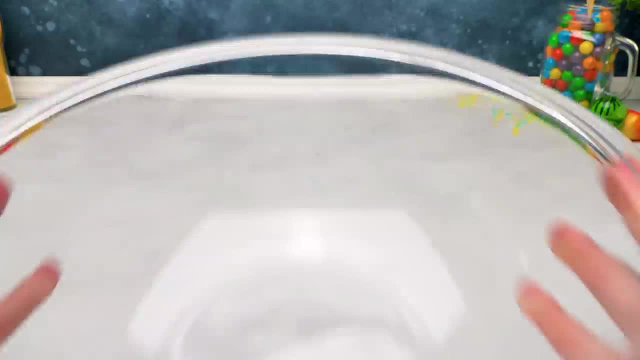 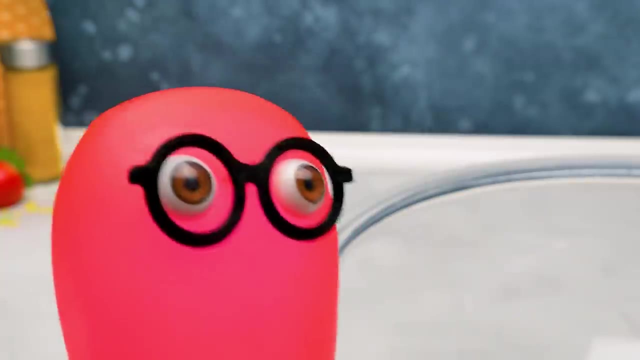 Bye cake. I'm gonna miss you Bye. In the meantime, we'll make a transparent cake. Let's make a transparent lemon jelly. Mmm, lemon jelly's one of my favorites. You go in the bowl, So look, I helped. 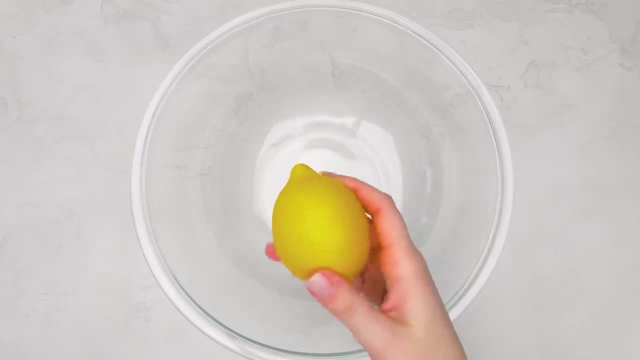 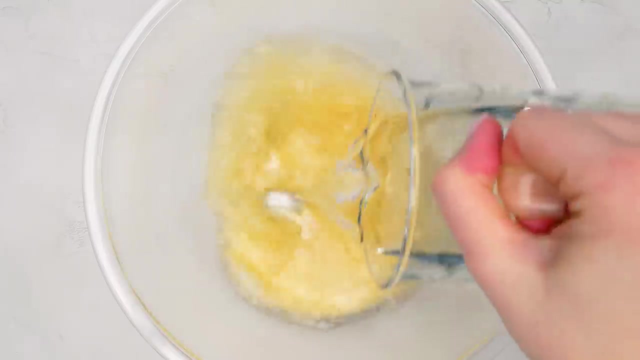 Sam, it's too early for the lemon. First, we need to make the gelatin mixture. We'll take 75 grams of powdered gelatin and add 375 grams of warm water to it. Now let's mix it properly like this: 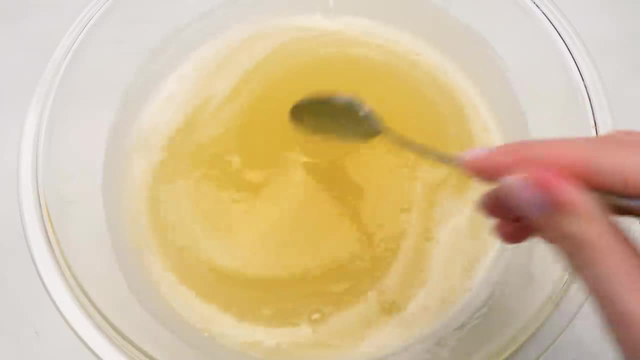 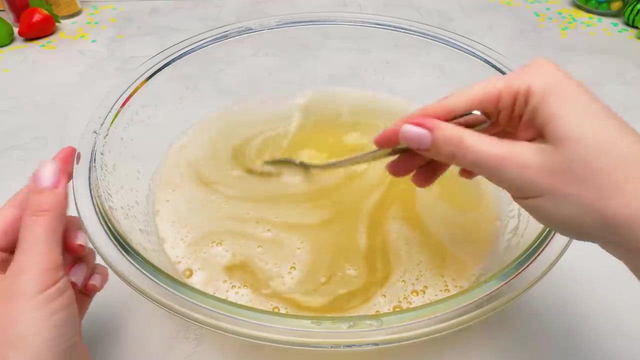 Susie, it's not that I mind waiting, but when is it time for lemon? We're close, Sammy. We'll add some sugar and lemon juice. So it's too hot. Won't it ruin the cake? It should be hot. 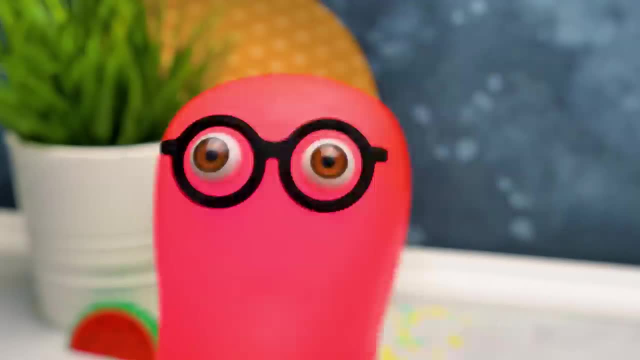 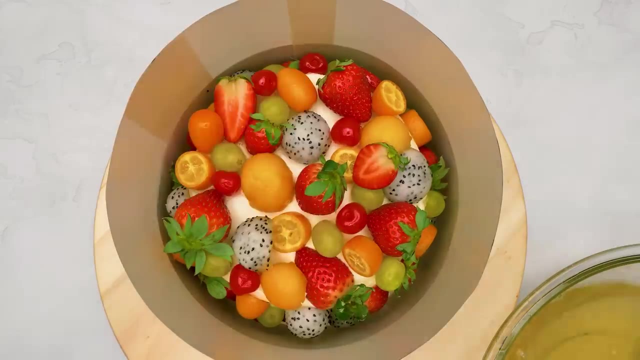 When it cools off, the jelly will become solid. Uh-oh, then I better move away. The cake is here. Are we gonna fill this thing with jelly? Yeah, we'll fill it up. The more the better. Oh, what if it pours out? 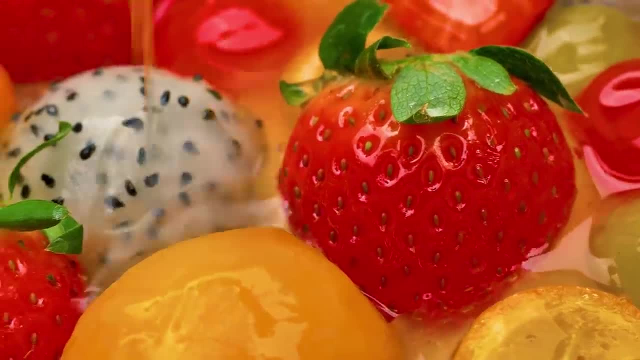 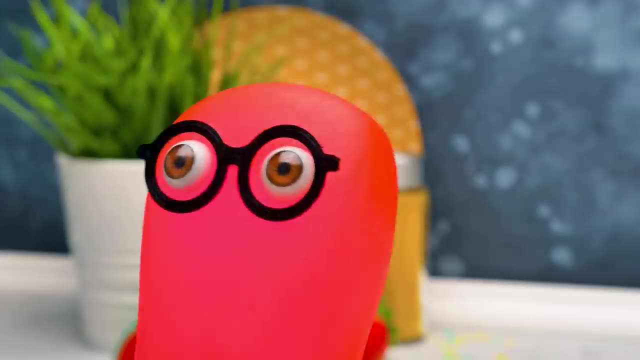 Sue, be careful. I'll do my best. Sammy, It's almost done. Let's just pour it over the fruit as well. I don't want to lose it. I don't want to look. Just tell me when you finish. 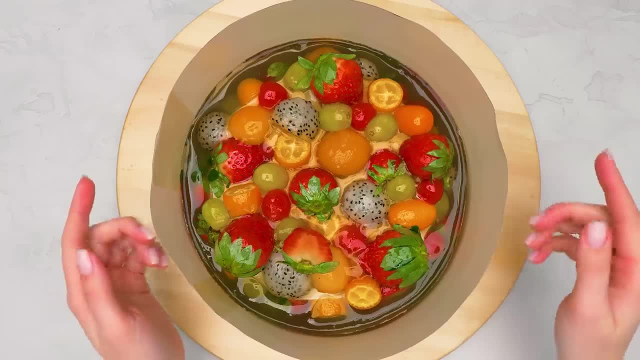 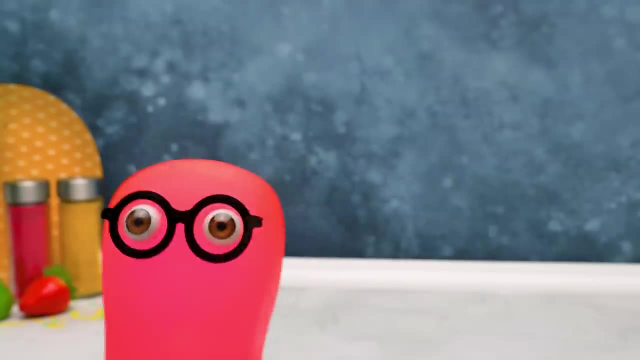 Sammy, it's over, You can turn around. The last step is to wait while it cools down in the fridge. Fridge again. For how long? Hmm, let's see. I think two to three hours is enough. No. 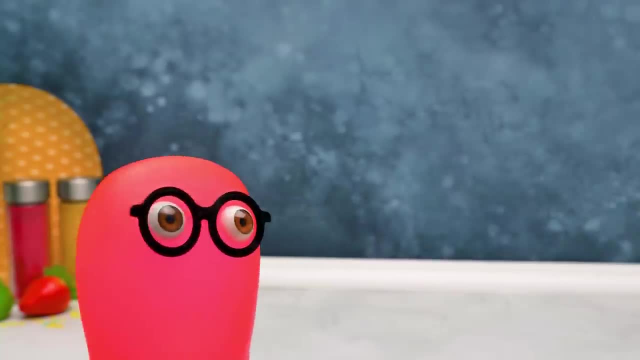 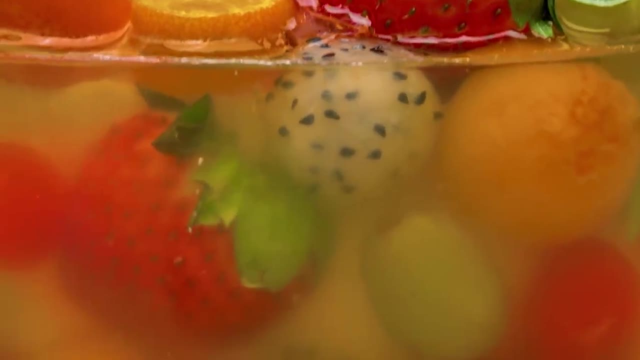 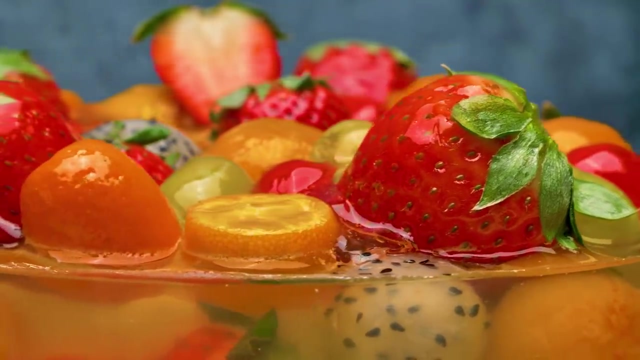 Sammy, it'll definitely be worth your time. Want to check out the final result? Follow me. Voila, Here is our masterpiece. Finally, the moment has come. I'll taste the fluffiest jelly cheesecake in the world. Just wait a second, Sammy.